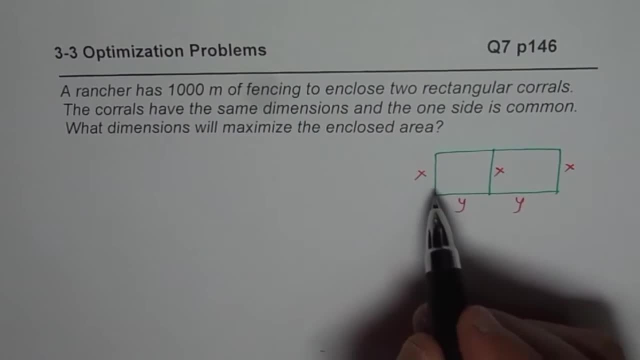 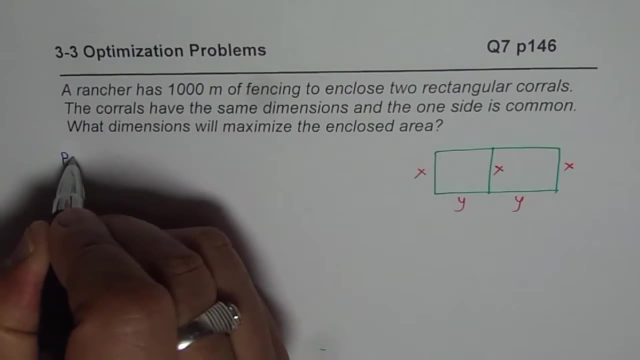 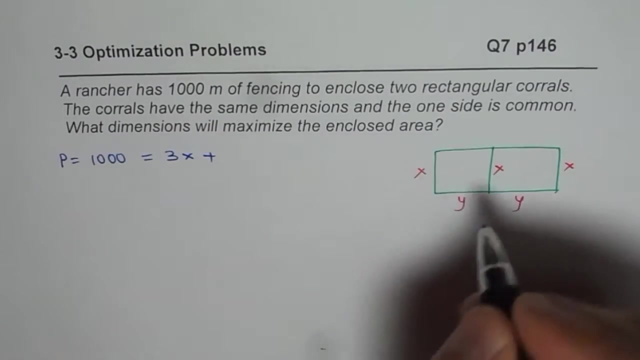 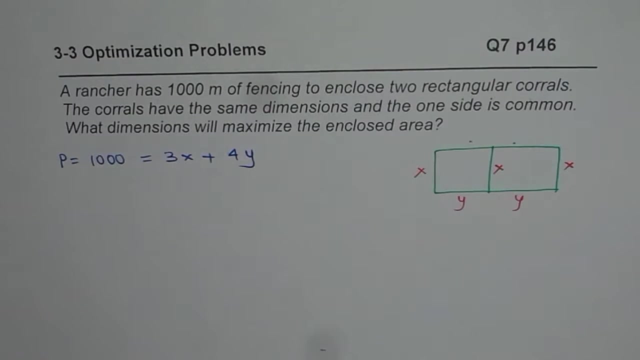 meter of fencing. That basically means that some of all these sides- that means there is 2y 3x, right? So we have perimeter, which is equals to 1000 meters- should be equals to 3x plus 4y. Do you see that? 4y? So that is how we can relate, both the things right? So 3x plus 4y is how we can relate. 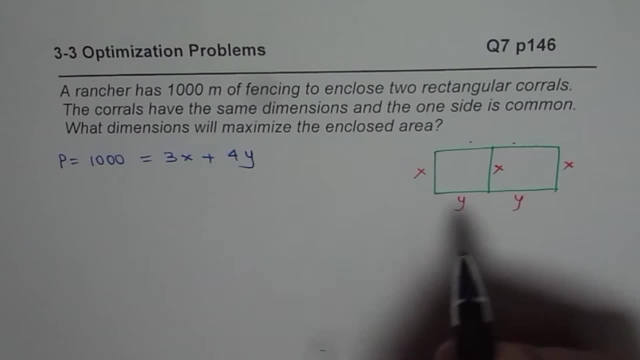 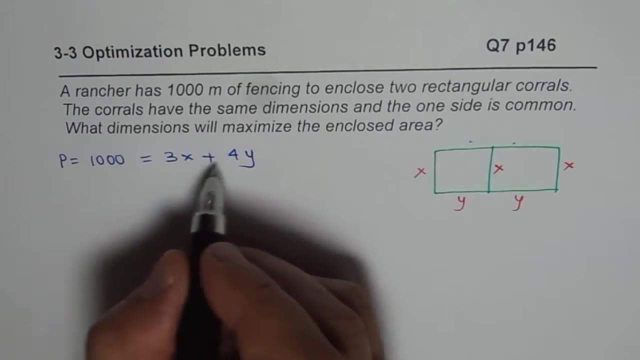 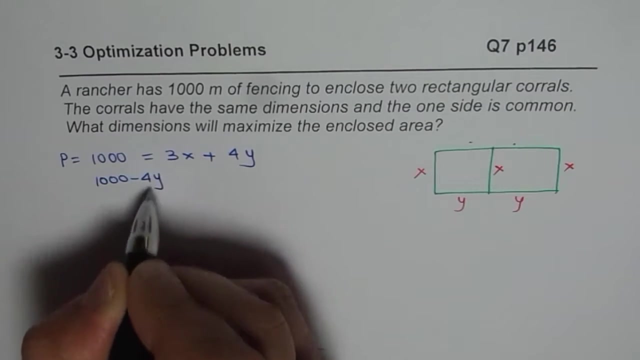 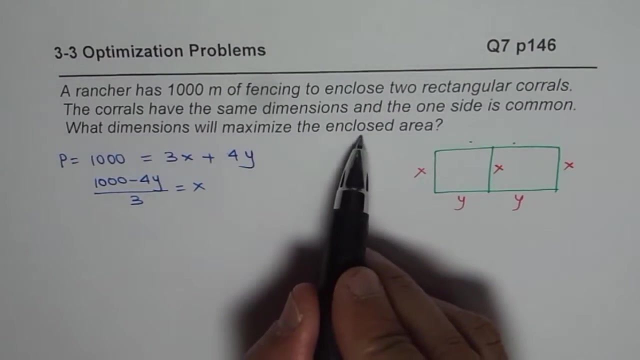 all these sides right Now. in this particular case, you could write one variable in terms of the other. For example, you would say that x is equals to 1000 minus 4y divided by 3. So that is the value of x. Now you need to maximize the enclosed area. So we say area will be length into width. 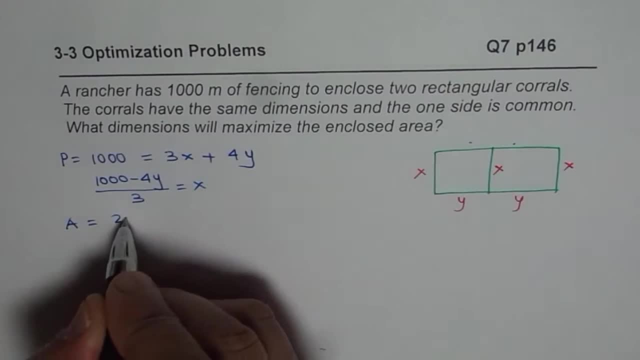 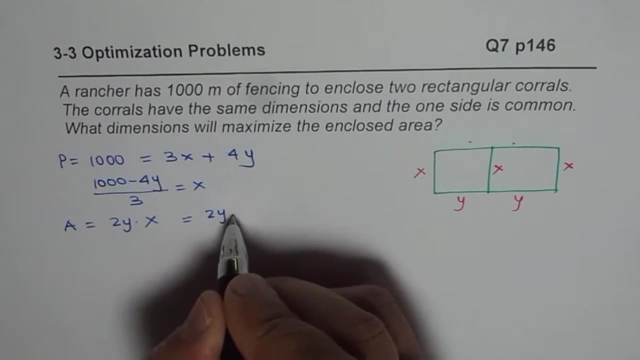 Now, length for us is 2y, right? So length for us is 2y and width is x for us 2y times x. So what we will do is, instead of x, we will write this expression, which we have got in y, So we can now write this as 2y times 1000 minus 4y over 3, right? So we got one expression in y, So we can say: area in terms of y. one particular dimension is: 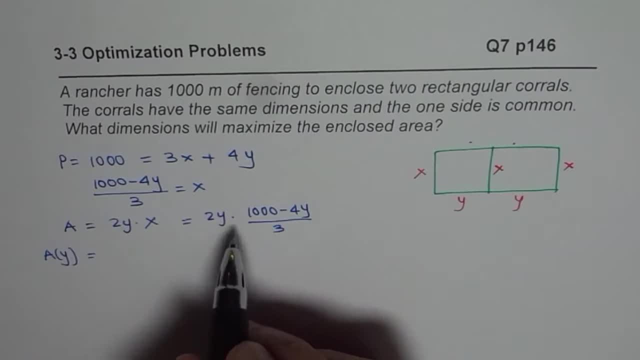 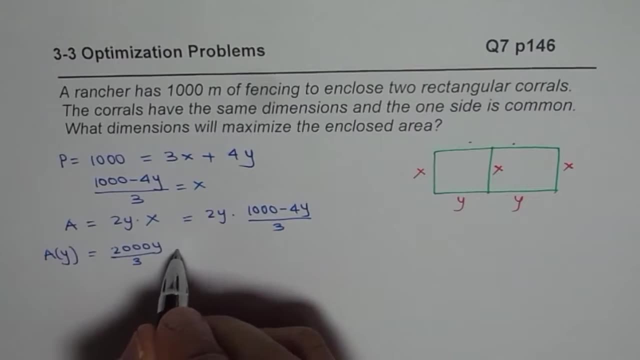 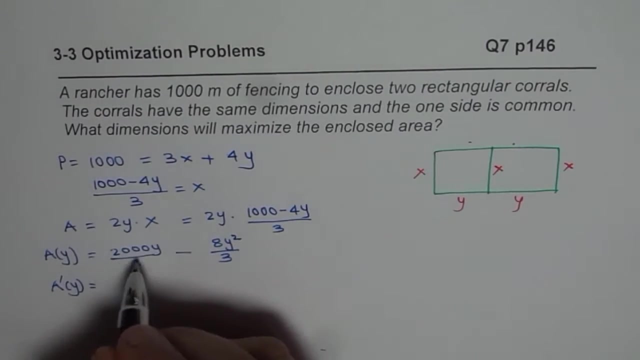 all this. So let us open the brackets. It is kind of simple, right? So we get 2000 y over 3 as the first term, and then the second term will be 8y square over 3, right? It is not a bad idea to actually to expand this and then find the derivative, since we need to find the critical number. Derivative for this is 2000 divided by 3 and derivative of this term. 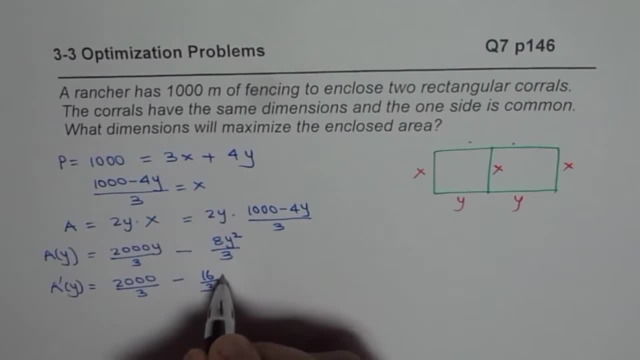 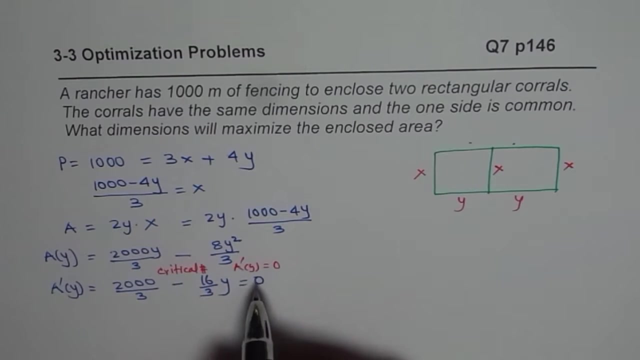 will be 2 times 8, which is 16 divided by 3, y, And for a critical number that has to be 0, right? So this is for finding the critical number, So we need to find critical number. So that means the derivative should be equal to 0, right? So that helps to find the critical number for us right Now, in this particular case, if you solve So we have, we can solve it on the right side also, or you can solve it on the left side. 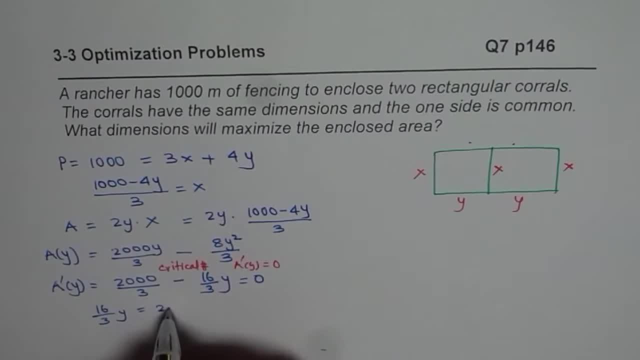 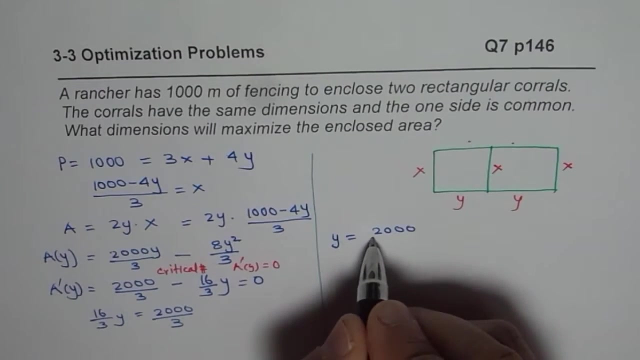 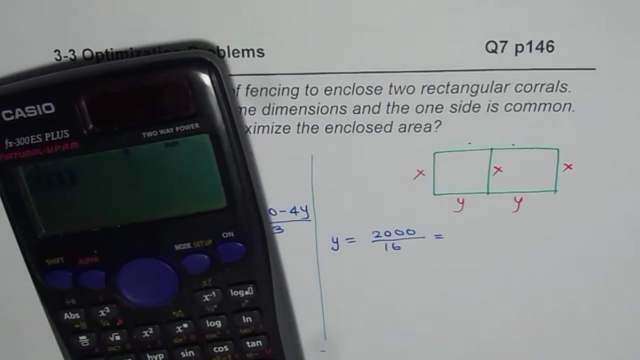 So we can say: 16 over 3, y should be equals to 2000 over 3, right? So now we will solve this on the right side of the page. So what we have here is that the y value should be equals to 2000 divided by 16, right? You can use the calculator to find the answer. So it is: 2000 divided by 16 equals to 125. 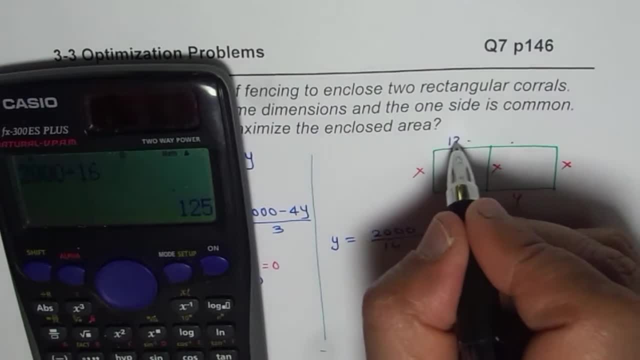 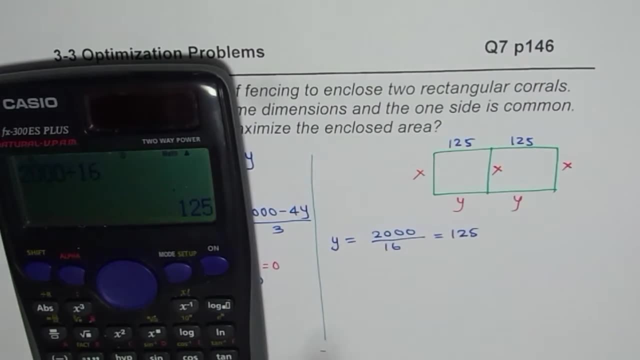 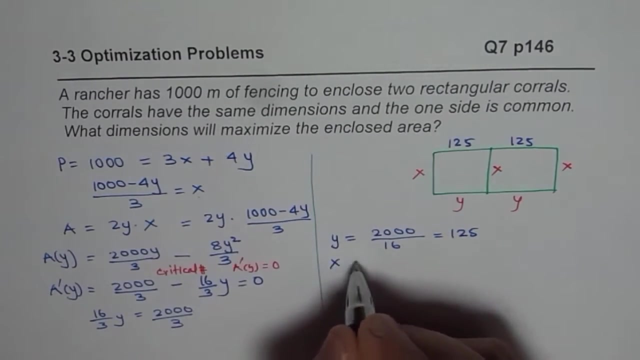 now, that is this y. that means 125 here and 125 here. so 125, 125 gives us 250 along the length, correct? so that is the y value. as far as the x value is concerned, we can find x from the expression here, which is 1000 minus 4 times 125 divided by 3, right? so that is equals to: let's 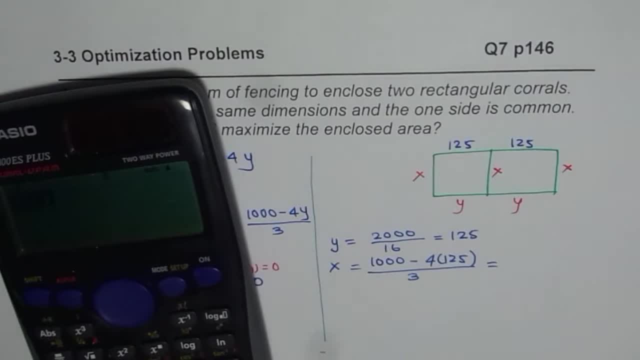 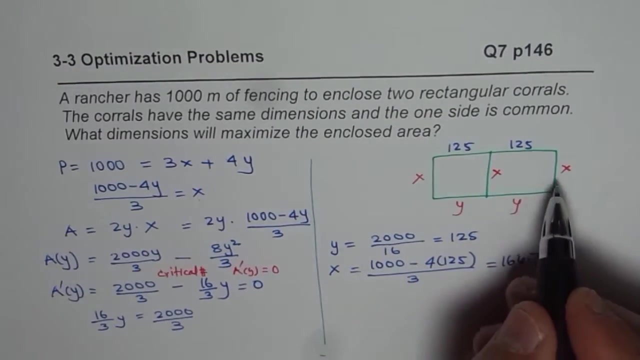 calculate this also: it is 1000 minus 4 times 125 and then you divide this by 3 to get the answer. in decimals it is. you can write this as 166.7, correct. so that becomes 166.7. the x value: right. so it says what dimensions will maximize the enclosed area. so in the 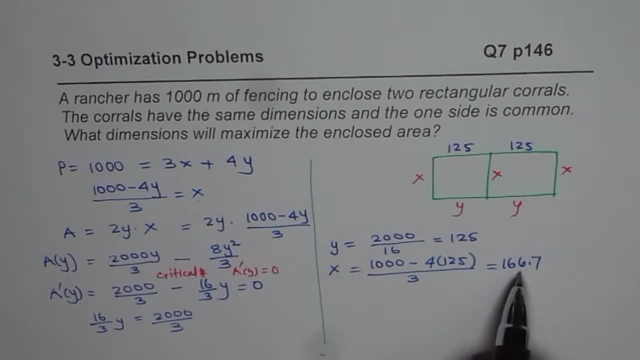 given diagram, y is 125 and x is 166.7, right? so that is how you can find if you need to find maximum area. let us say, if you need to find. if suppose in your test the question is to find maximum area, then your maximum area will be 2 times y, 2 times 125. 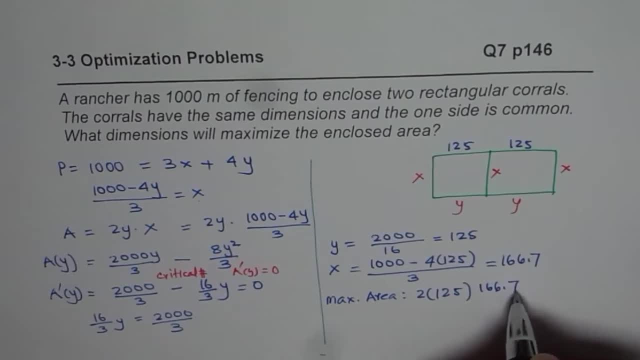 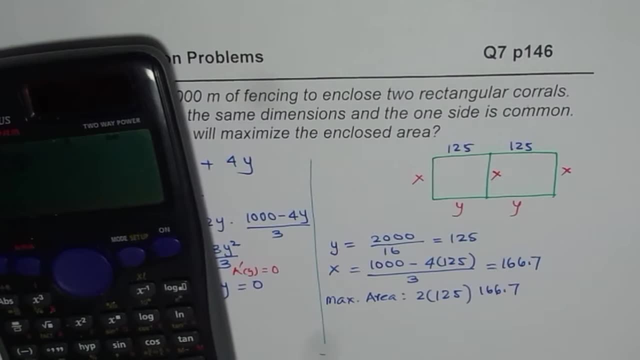 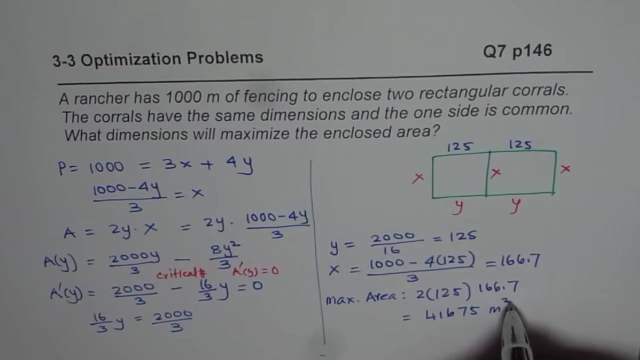 times the width, which is 166.7 right. so that will be: let's multiply 2 times 125 times 166.7, so approximately that is going to be equal to 416, 75. the units are meter square right, so that is approximate value for the area. maximum area is 166.7 right. so that is how you can. 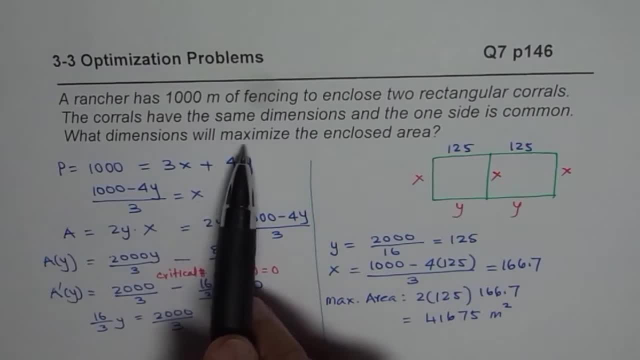 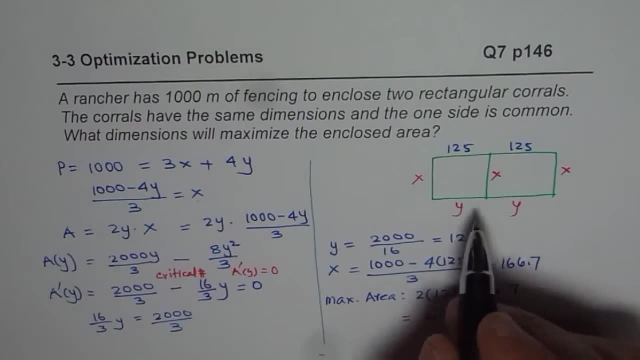 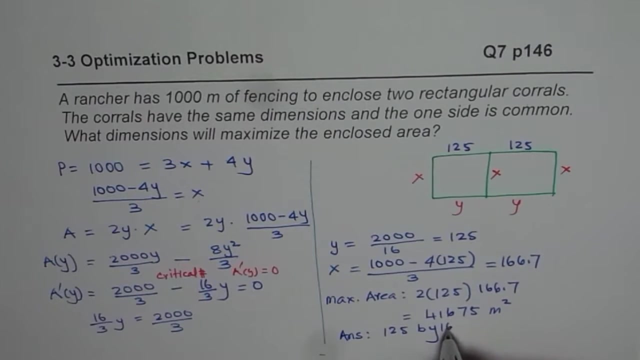 calculate the maximum area, right, but the question is what dimensions will maximize the enclosed area? so you can say that the length is 150, so each, you can say each corals will be 1, 5, 125 by. so it be. so you can write answer as 125 by x is 166.7 each. you understand so. so both are the same. 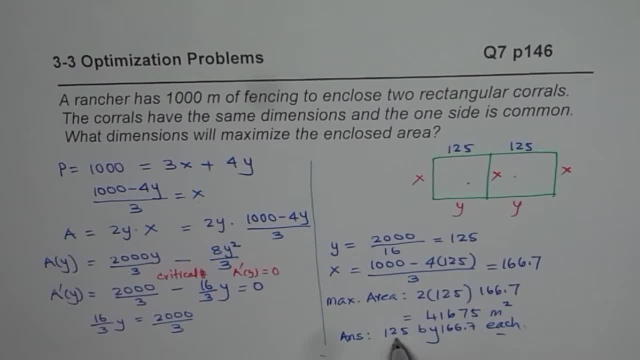 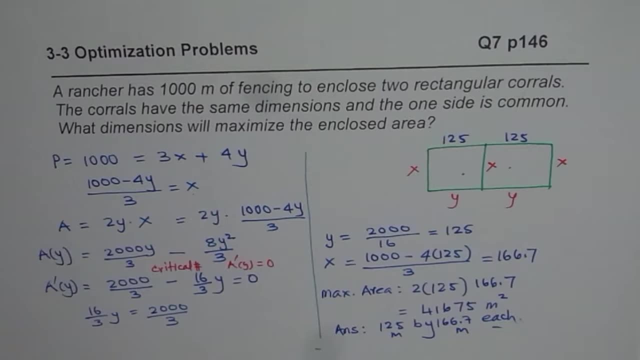 right, so 125. by this, and the units are in meters, you get the idea right. so it is each. so that might be creating a confusion for you. so that is how you should be solving this particular question right. as far as the boundary conditions are concerned, you can actually use this relation to find the 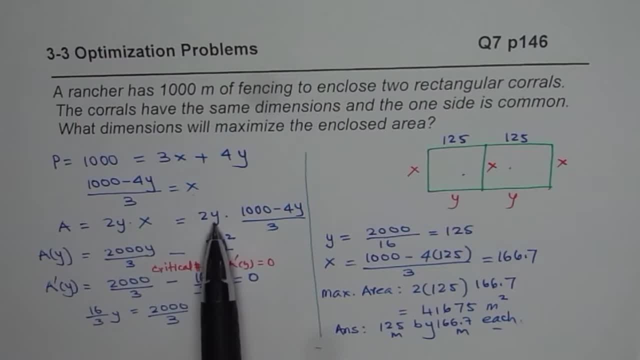 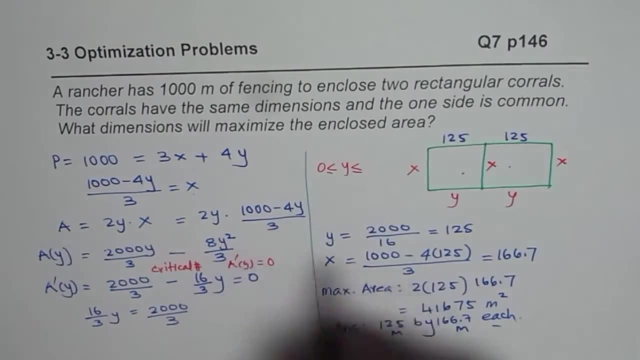 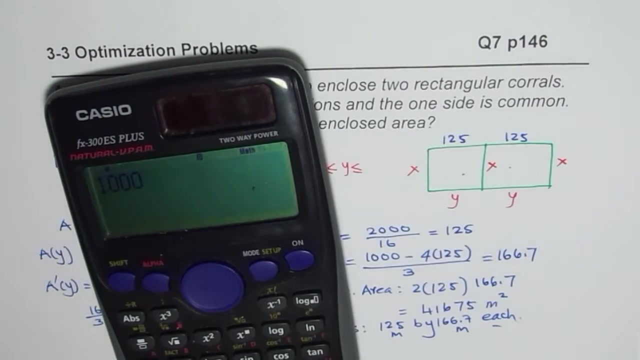 boundary conditions correct. so y value could be zero. so the boundary conditions also, you can test. so y for you is greater than equal to zero and this cannot be negative, right? so 1000 divided by 4, so 1000, you know half is 500, 250 is your answer. anyway, let's divide 250, right? so y values between. 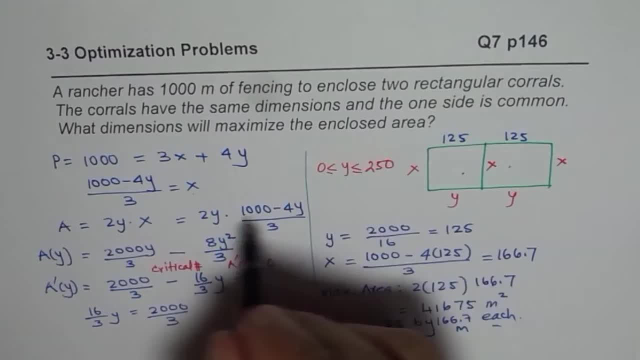 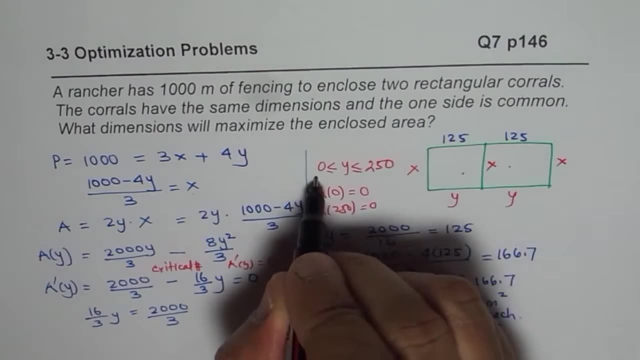 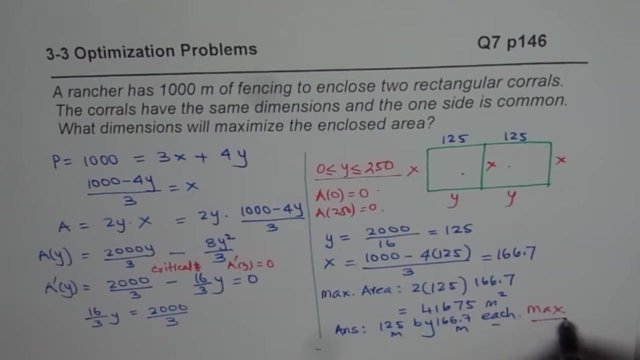 1000, 0 and 250, but any value put so a of 0 will be 0 and a of 250 will also be 0. so these boundary conditions will always give you that result. therefore, you, the answer gives you maximum area. so it's also important to mention this in your solution. so